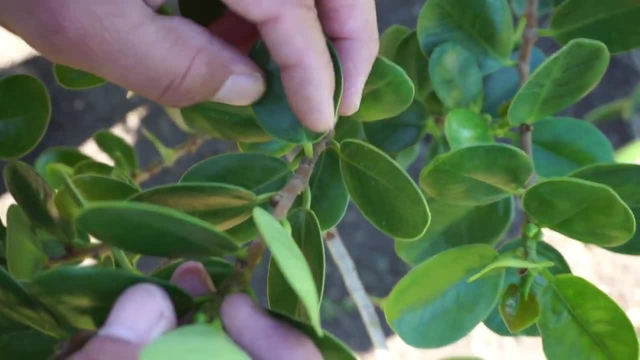 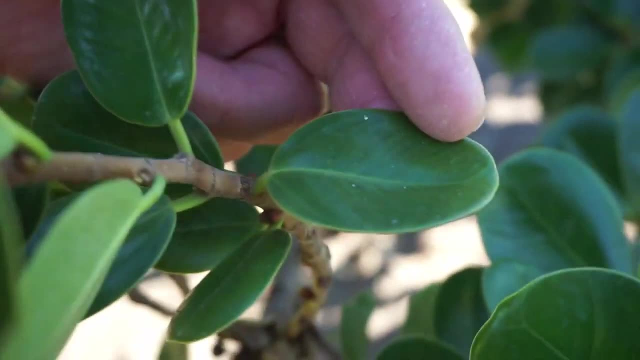 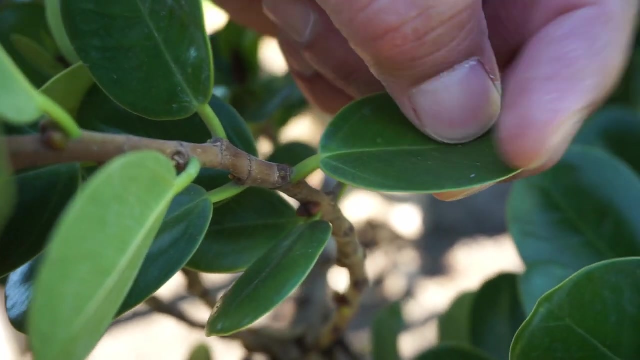 and you'll find it by going to where the buds are, you know, and you'll see that that's the simple leaf structure and it is a rounded leaf And the same with the other. you know, you have the margin, the petiole, the swell, you got the midrib in this area and here are the veins. 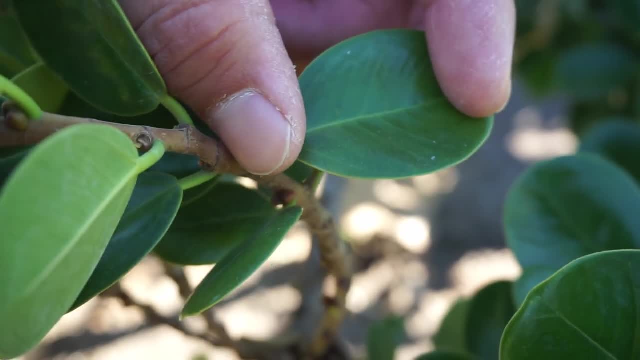 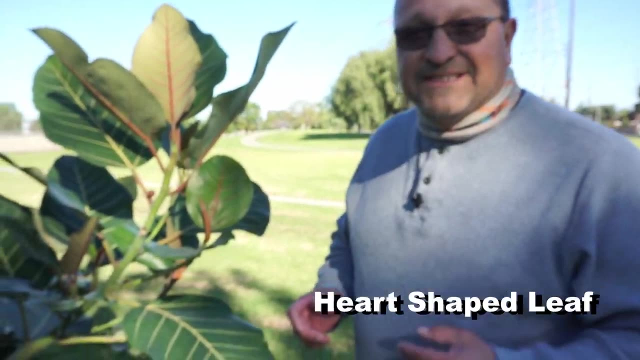 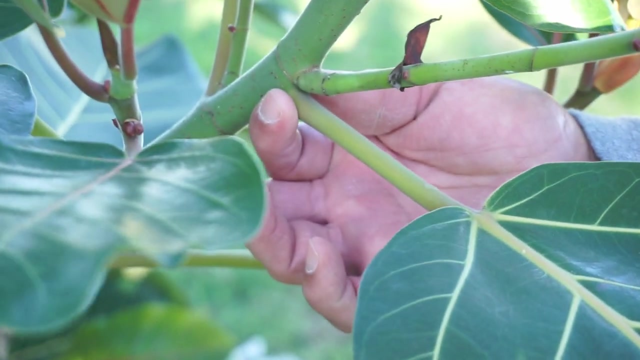 And well, there's no tip, but this is what the leaf tip would be. This is an example of a rounded leaf shape. So right here we have a simple leaf and it's a heart-shaped leaf. So you'll go back to where the petiole begins. So this used to be a bud and you could see the swell. So this is the. 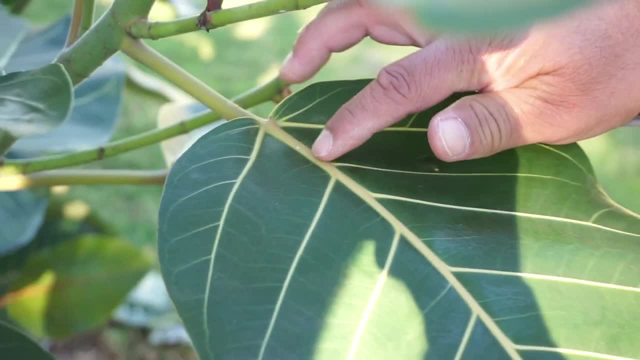 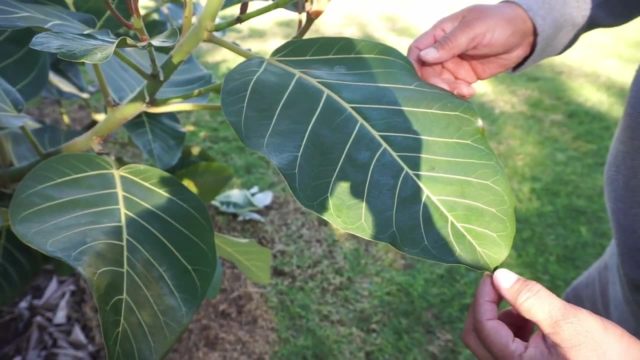 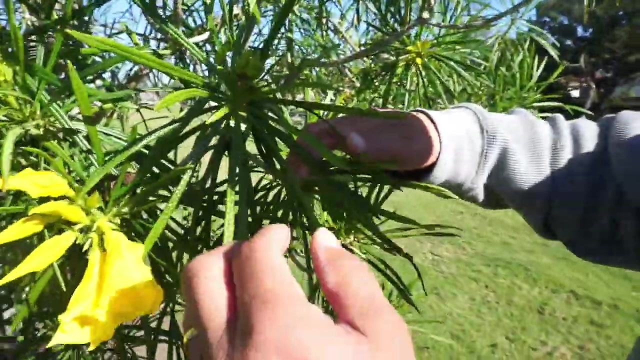 leaf. Here's the petiole. You have the midrib, You have the veins, You've got the leaf margin and the tip, And then this is a heart-shaped leaf. So here we have a simple leaf, and this leaf shape is a lance-shaped leaf. 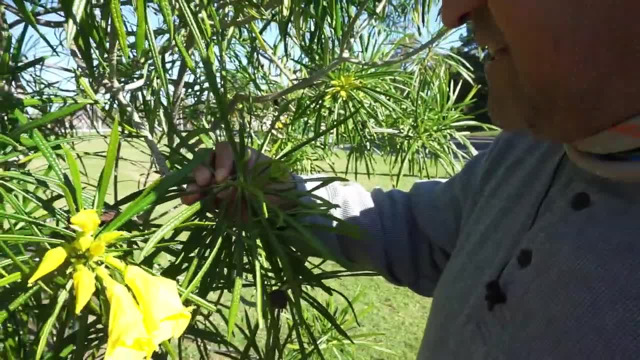 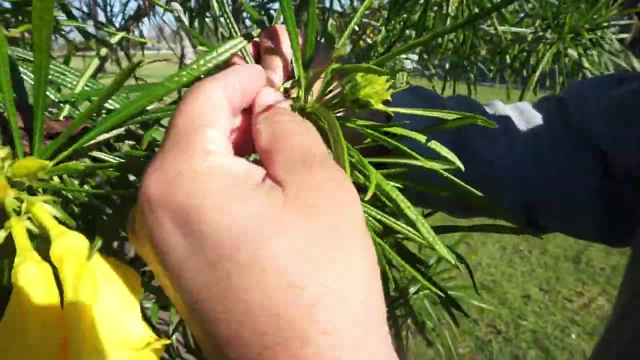 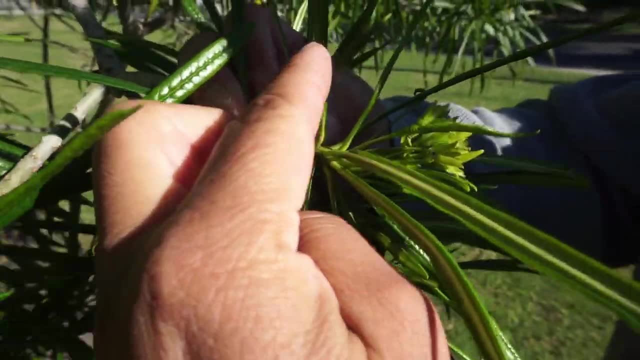 And if you saw our last video, we talked about phylotaxy and leaf arrangement on a twig, and that's what this is. It's all a world arrangement. Anyhow, to see that it's a simple leaf, you'll go to the bud. You'll see the petiole here And then here's the margin: You got the midrib. 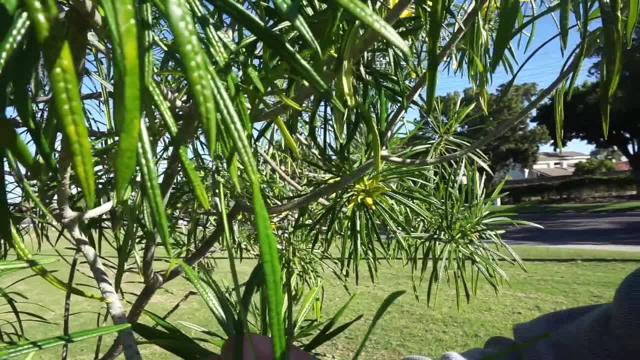 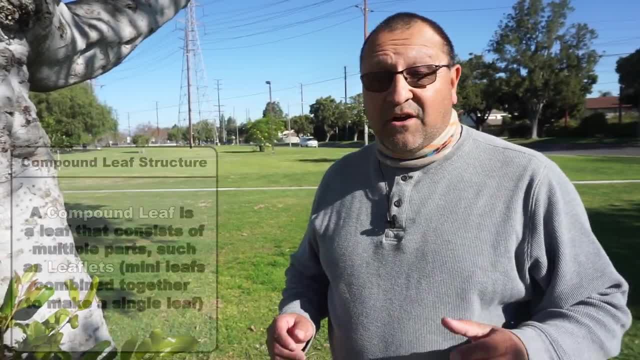 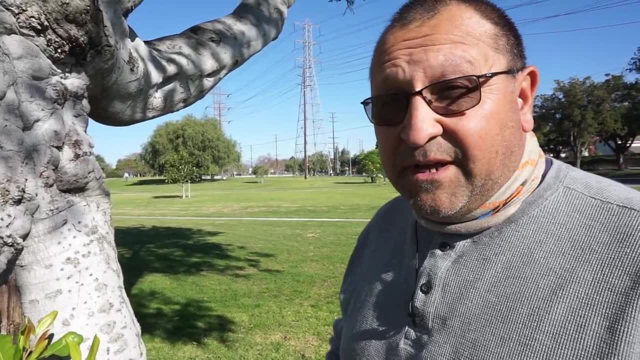 and then the veins inside, And then here's the tip. This is a lance shape. Some people may call it a lanceolate. What I wanted to talk about next is compound leaf structures, So the first one I want to talk about is one called a pinnate. They also call it once pinnate, So this is how you'll. 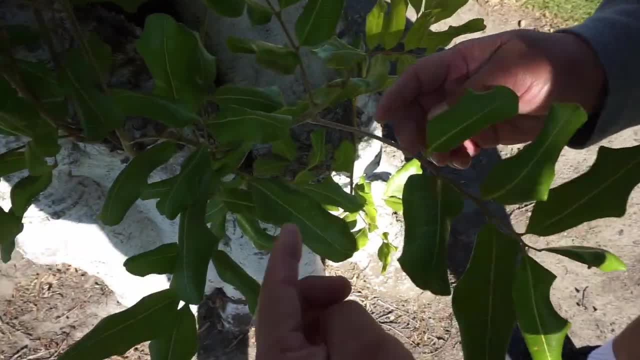 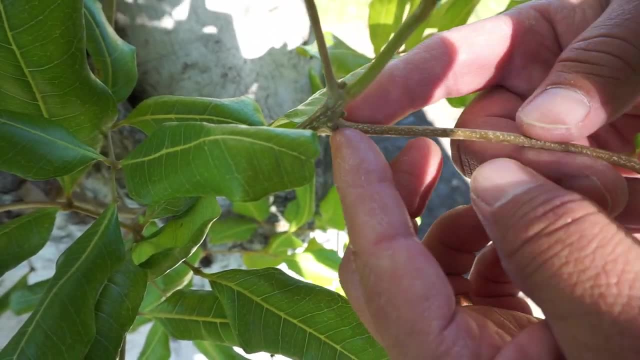 find a pinnate leaf And remember it's a compound leaf. So you go to where the petiole is and you're going to follow that up to where the bud is And where this swell is. this is where the leaf begins. So this is the petiole. Now 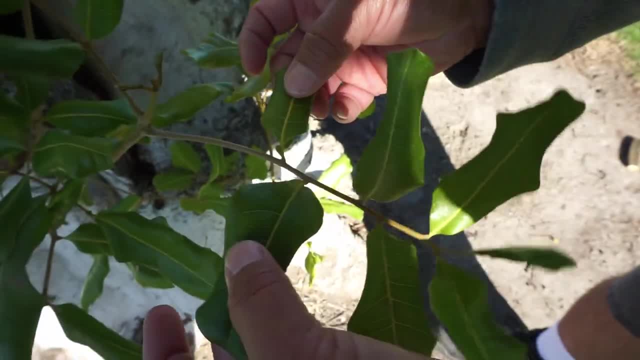 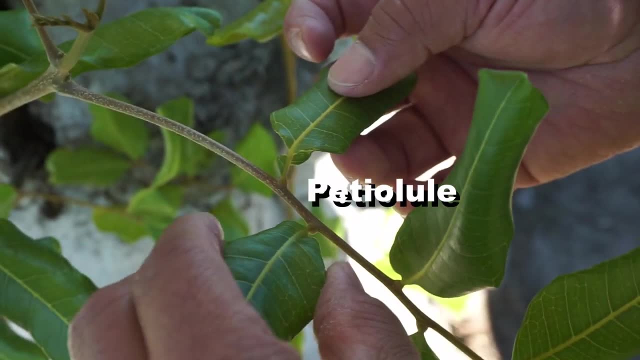 if you're going down the leaf, these little pieces right here- they're not actually leaves, they're leaflets. And where it connects, these little pieces right here are called petiole lulls. When you go further down, this right here is called a rachis. 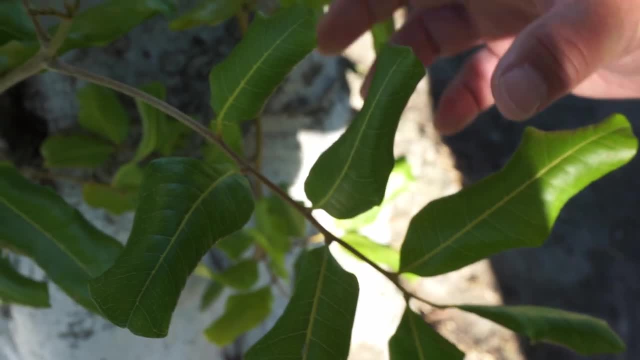 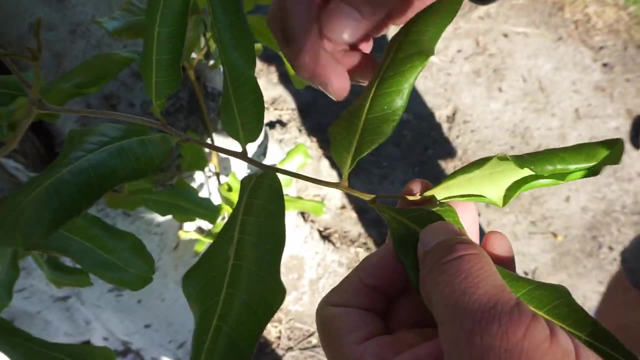 Now, that's part of the structure of a compound leaf. You have the petiole leaflets, petiole lulls, rachis, So this whole piece makes one leaf. You'll still have the same thing You've got. 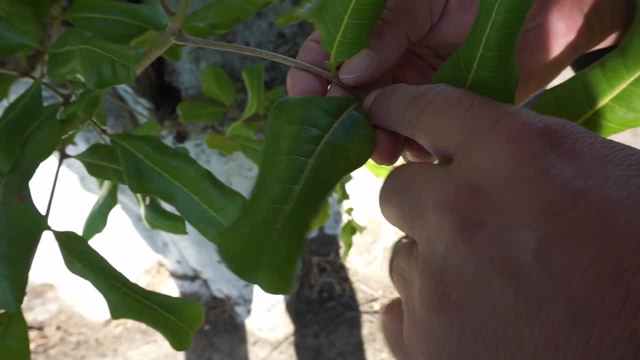 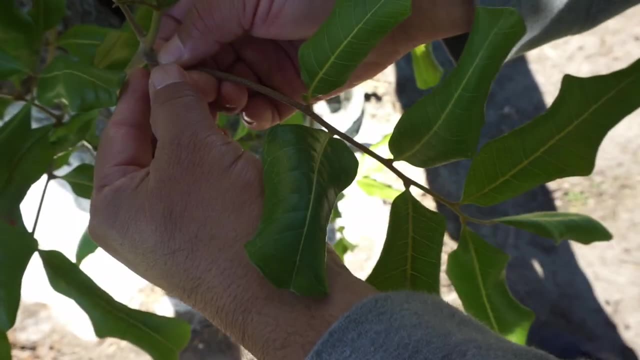 leaf margins here and then you've got a petiole lull, You've got a midrib and you've got veins and also a tip, But this is not the leaf. If you go back and you pop this off, oops, kind of popped. 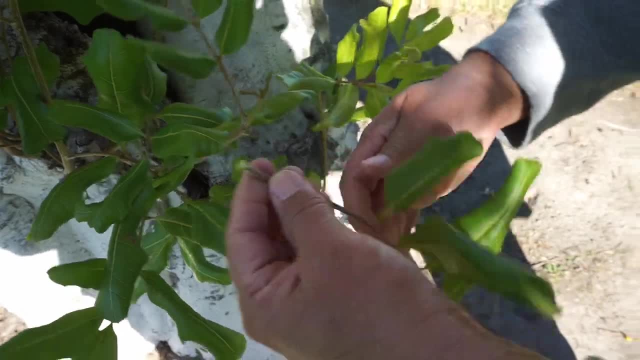 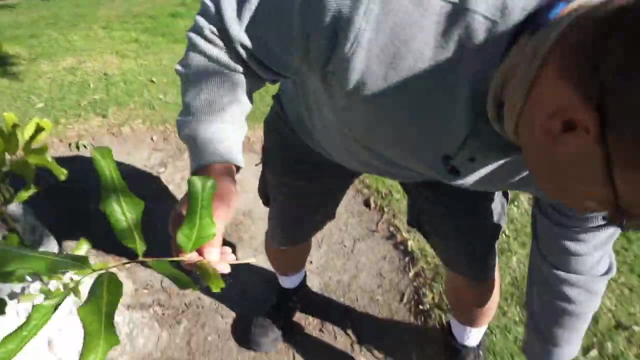 it off kind of crummy. If you go back and you pop this off, oops, kind of popped it off kind of crummy- This would be considered one pinnate leaf. So I'll get you another leaf here. This is also another. 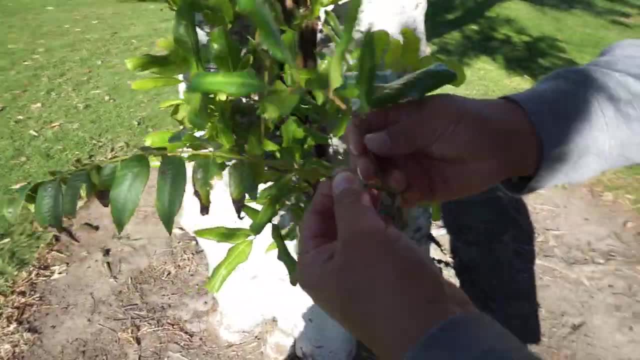 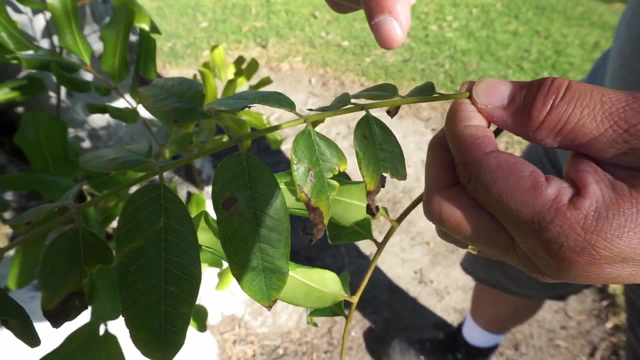 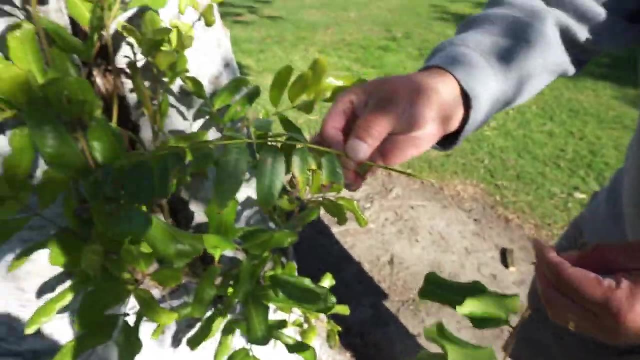 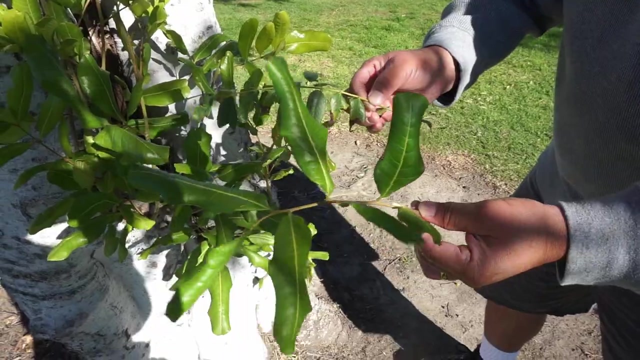 pinnate leaf from another tree. So you can see on this one where the swell was. Now you have the leaflets, You've got the petiole, lulls, the rachis. This is considered one whole leaf, Not these little pieces. And on this one, this is one whole leaf. This is a pinnate, or once pinnate. 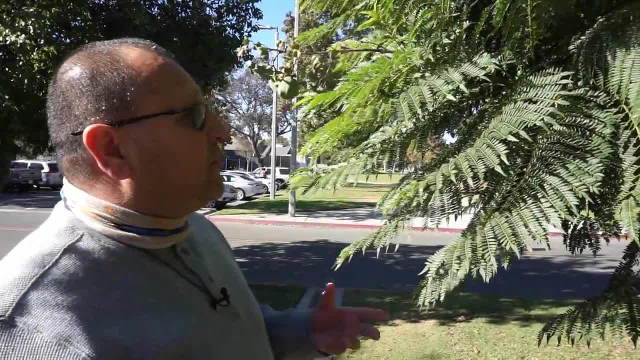 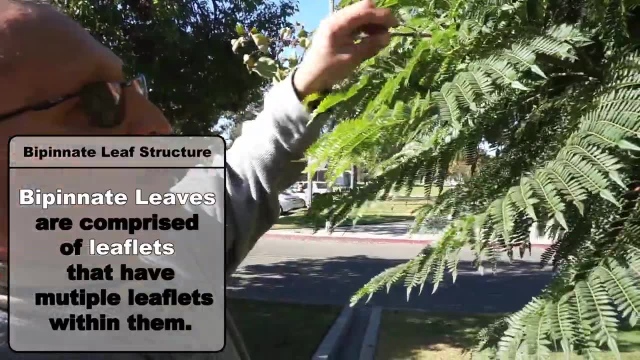 leaf, Both of them. Now, what I wanted to talk about was a bipinnate leaf, So the other one we talked about was a pinnate. So in a bipinnate they also call it twice pinnate, or you know. 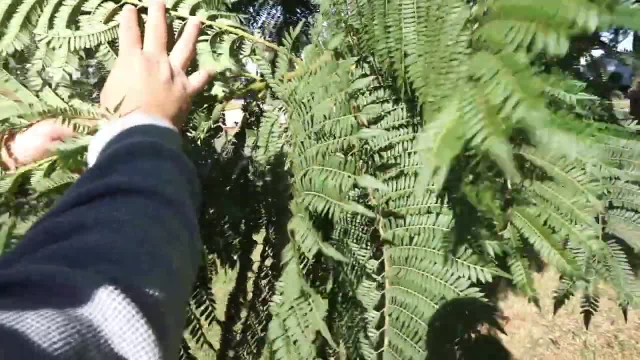 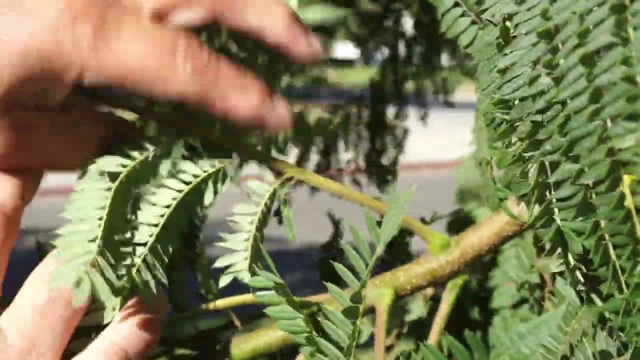 bipinnate. The way you would find that is: you'll go down the leaf, you'll find the petiole, you'll see where the bud is. This is a swell, So I'm going to switch over to this one. You. 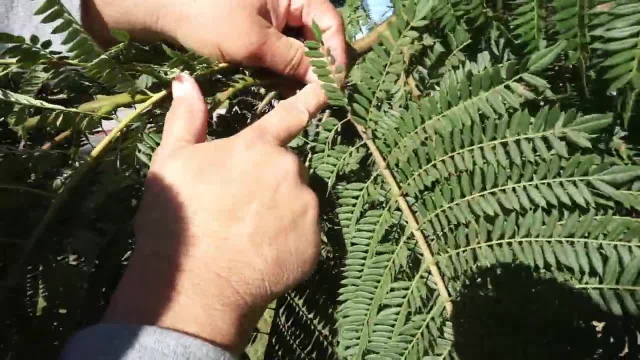 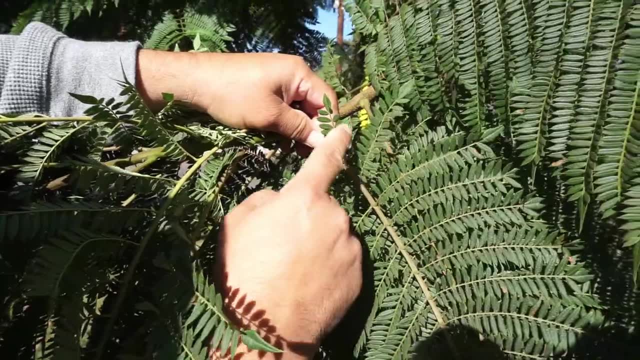 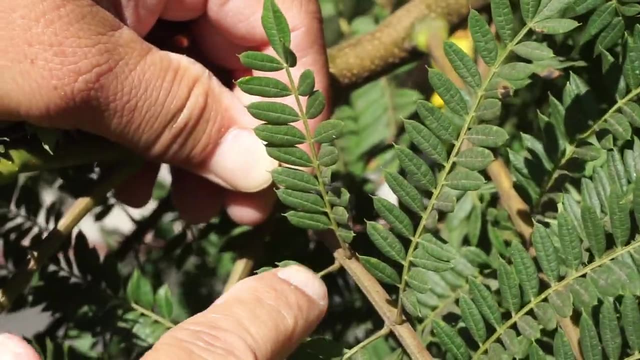 maybe see it better. So this is the petiole. Then you go up further, These little pieces. here are leaflets. On the pinnate one it was just a full leaf, But this leaflet looks like a, you know, like a pinnate leaf At this point, right here is a petiole lull. Then you got the rachis. 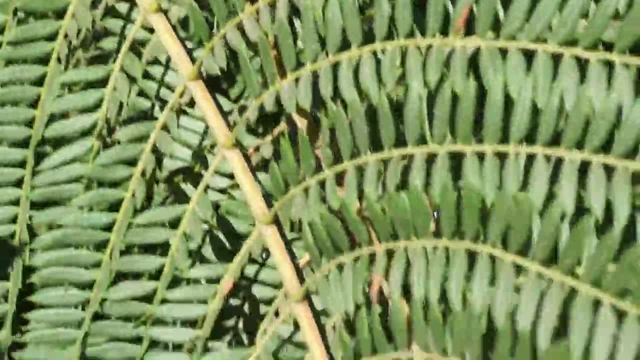 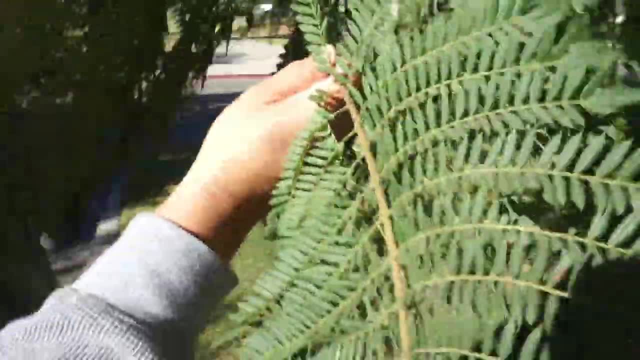 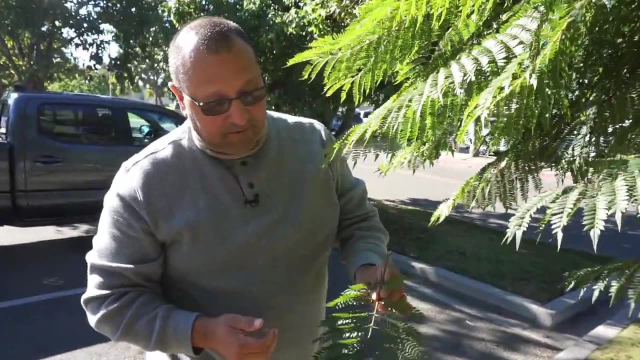 So this is the leaflet. You go further down, This is the entire leaf. So to find the leaf, you would pop it off at the bud swell. Now this is a bipinnate leaf, or twice pinnate, This whole entire leaf. 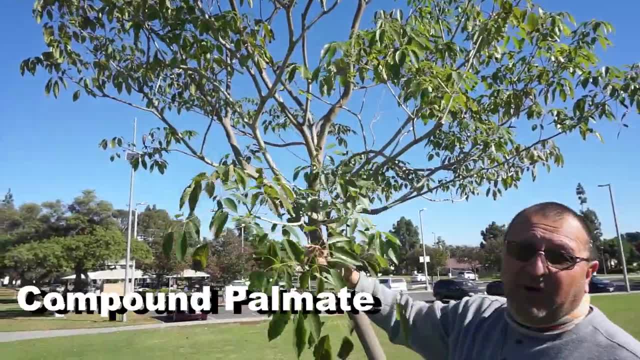 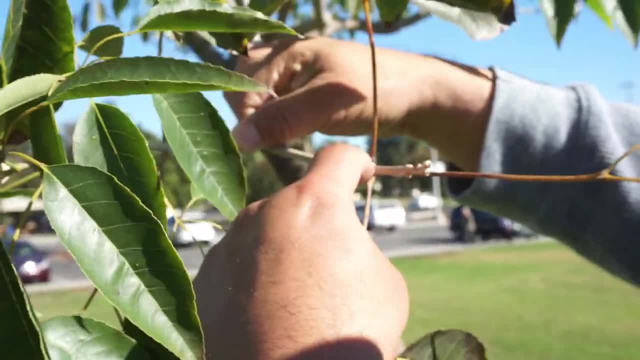 So what we have here is a compound palmate leaf. So you're going to know it: It's a compound palmate. by following the petiole to where it swells, You really don't see a bud. On this one, you could see the bud. 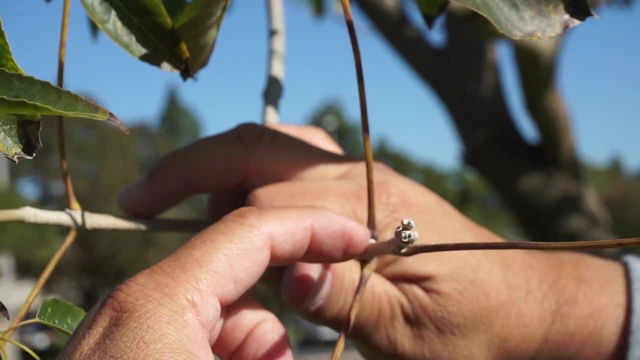 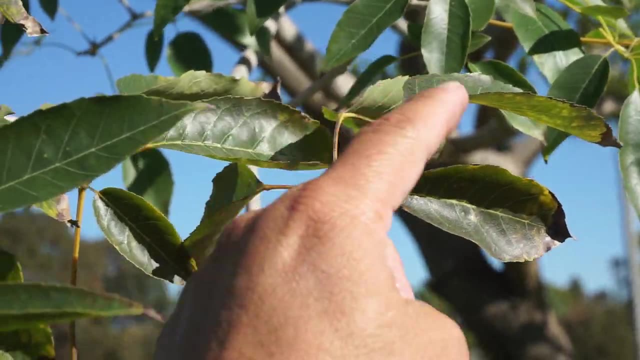 On this one it's really not pronounced, but you could see how the leaf swells. So this is the beginning of the petiole. So you follow that up and then you have these leaflets. So the same thing: petiololes and then the leaflet. 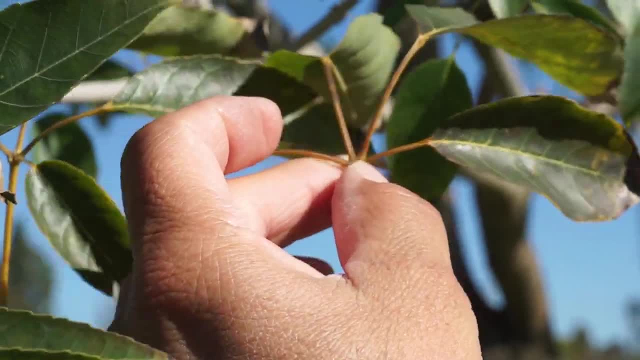 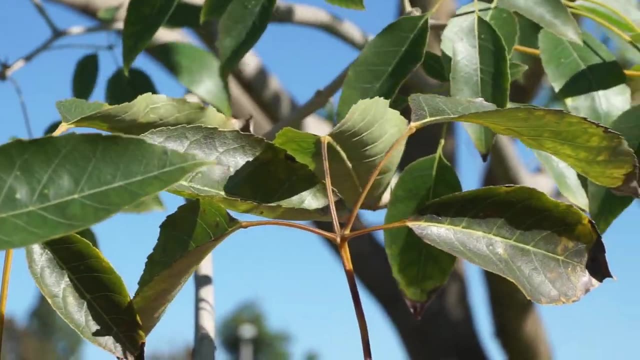 Looks like a simple leaf, but if you follow this here, they're not really swollen, they're straightly attached. You'll see the difference here how it swells And there's that abscission zone. So this right here, the way it's shaped. 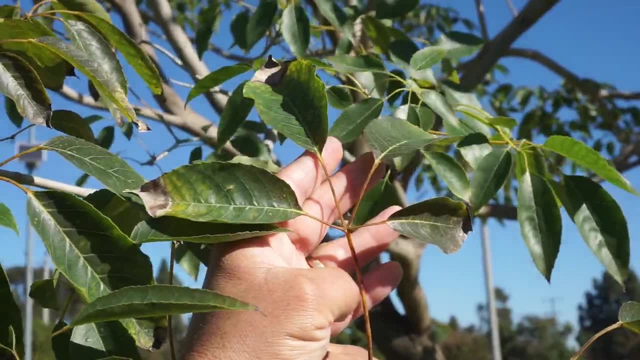 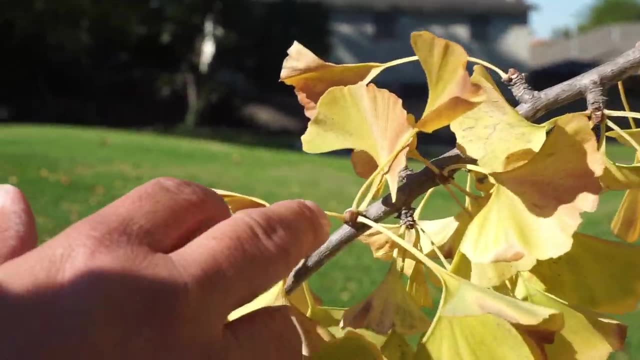 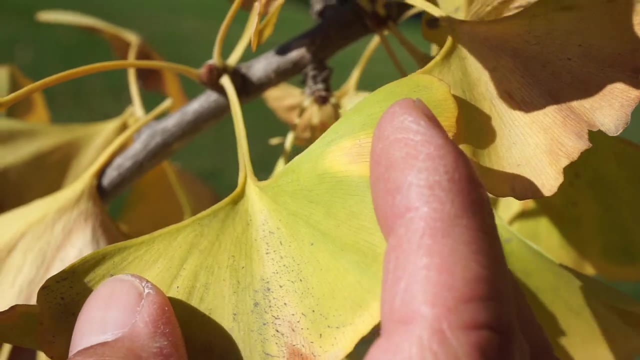 is a compound palmate leaf. Here you got an example of a fan-shaped leaf. So to find the leaf you'll go to where the bud is and right there where the abscission zone is. This is the petiole and here's the leaf. 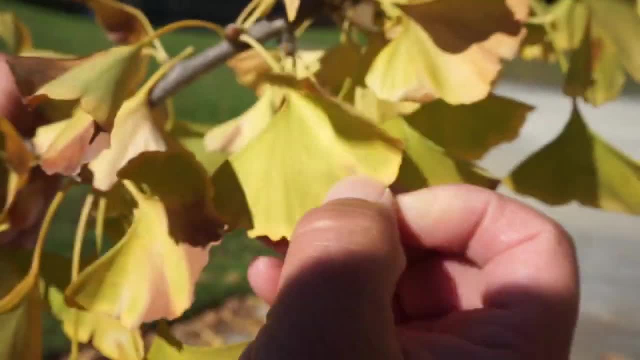 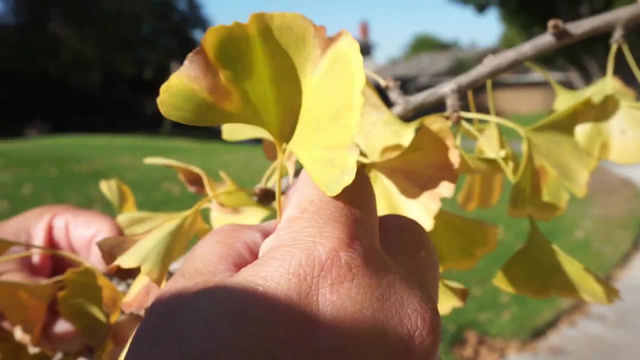 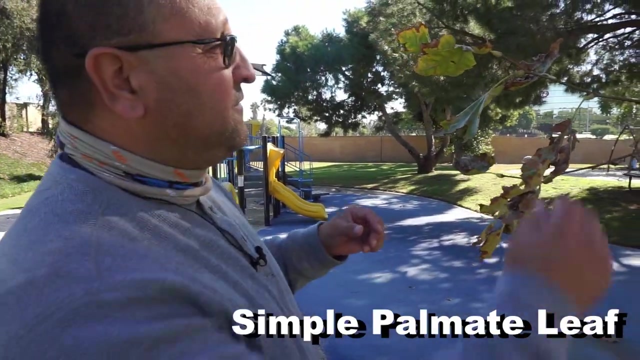 It's a little bit different. You don't really see the, the midrib that's parallel-veined. Anyhow, this is the entire fan-shaped leaf. It's a simple leaf. Here we have a simple leaf. that's a palmate leaf. 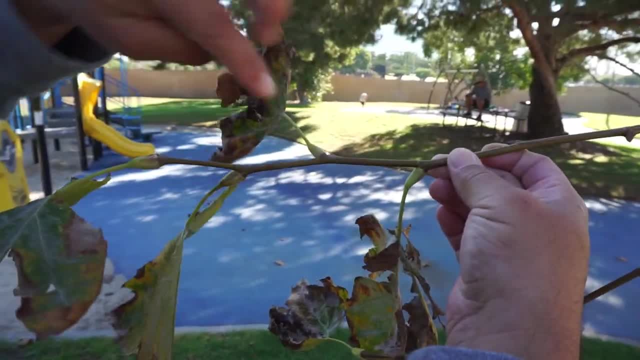 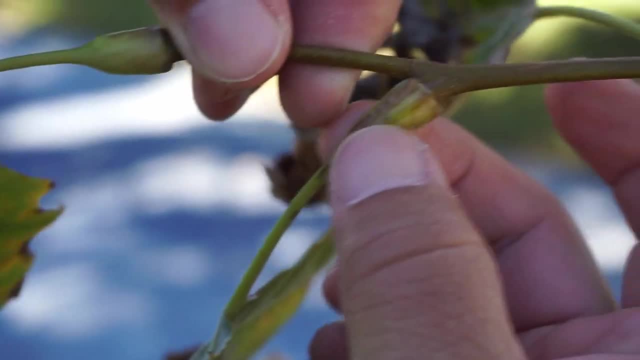 This one's really pronounced. So if you go to the stem you could see the swell here. I'll go to this one. it's actually bigger. So here's this petiole where it begins. That's the big swell section. 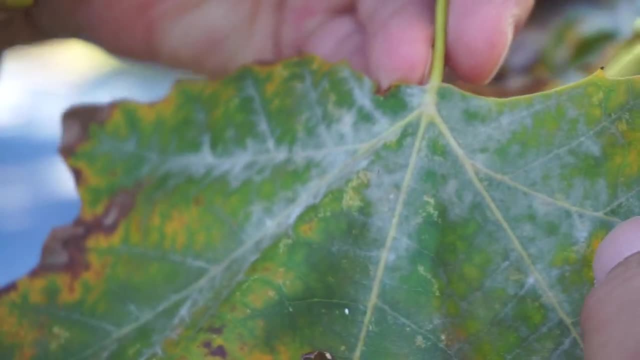 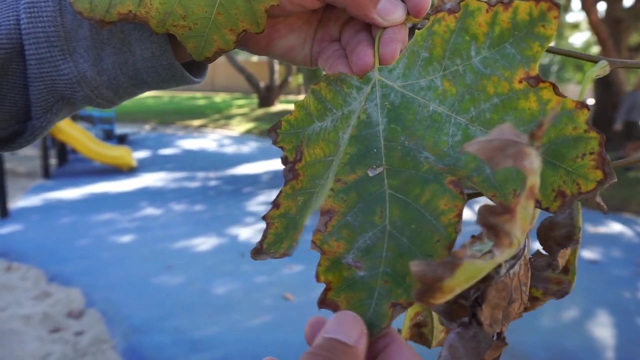 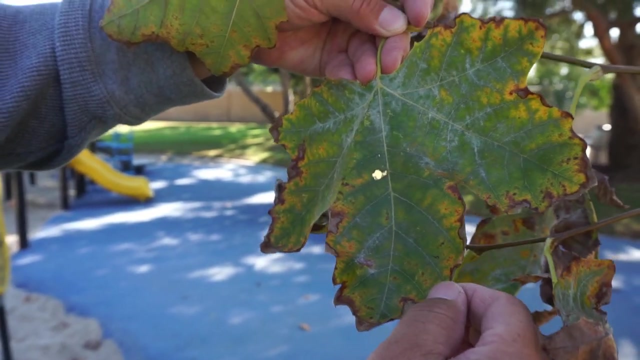 Then you got the petiole and then here starts the leaf. This is a lobed leaf. It's also a simple palmate leaf, So where you start here and then they all kind of fan out like a hand. this is a simple palmate leaf. 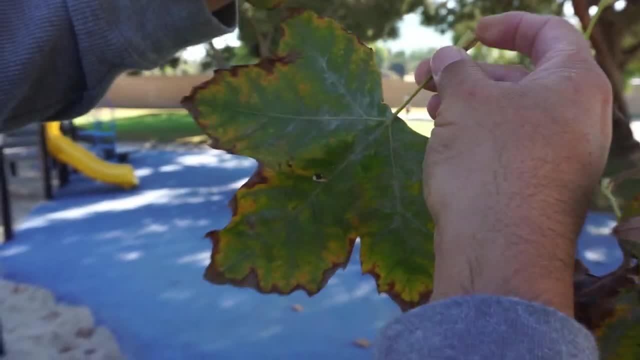 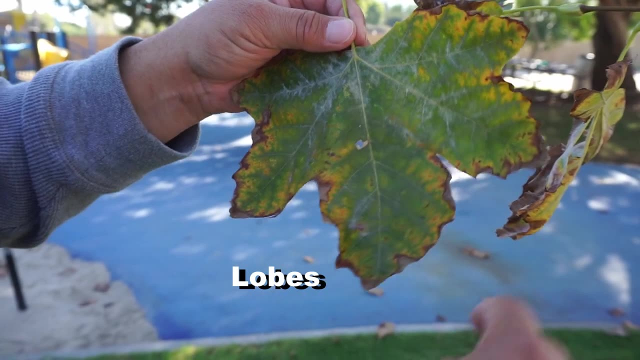 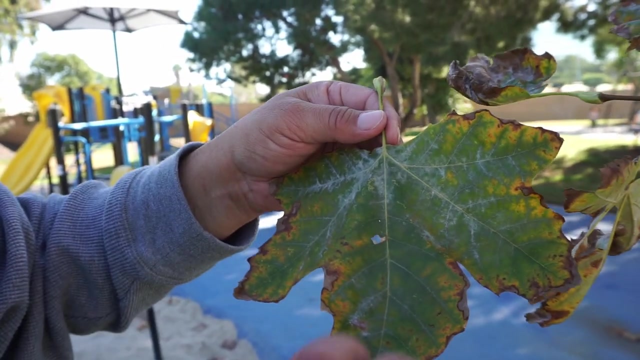 So you take this off and that is a simple palmate leaf. What is lobed? Lobed are these sections here Almost like fingers of a hand. So all of them have these almost like you see, these big little leaves, Unlike the compound palmate.